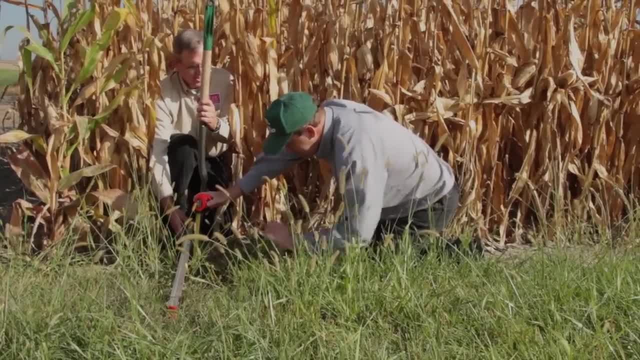 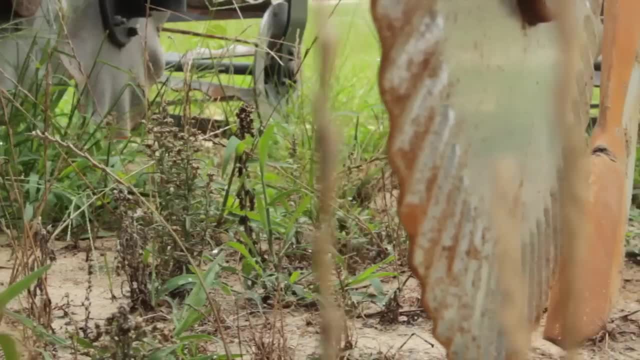 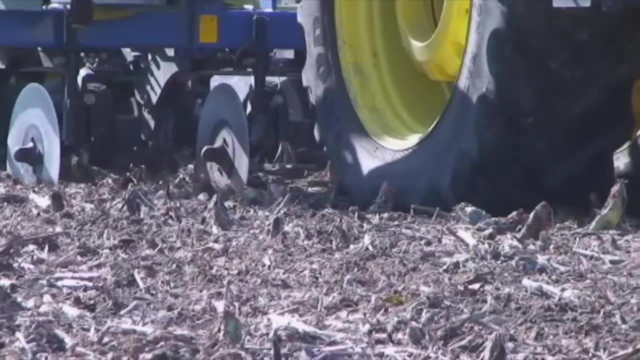 Ohio State, who use science to put conventional wisdom on its head. We're trying to tell the farmers that you cannot solve your problems with steel. You know, steel is shiny. You can put your hand on it. You can spend a lot of money on steel, And even with a subsoiler. 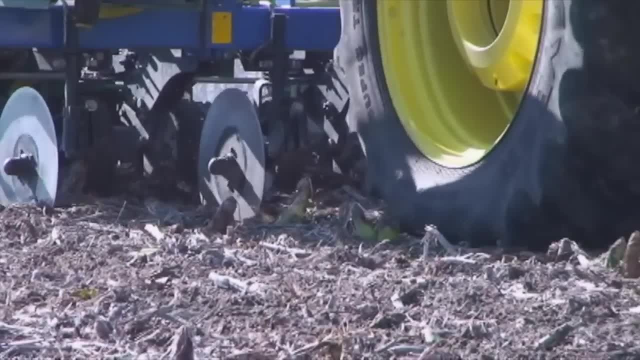 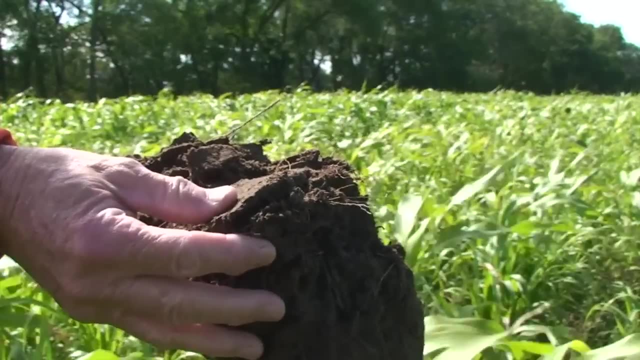 that may have minimal surface disturbance. it's really not solving the problem. You know we're seeing that soil structure can be better solved by using natural rooting systems through our cover crops or continuous no-till from the cropping systems. And we have some other. 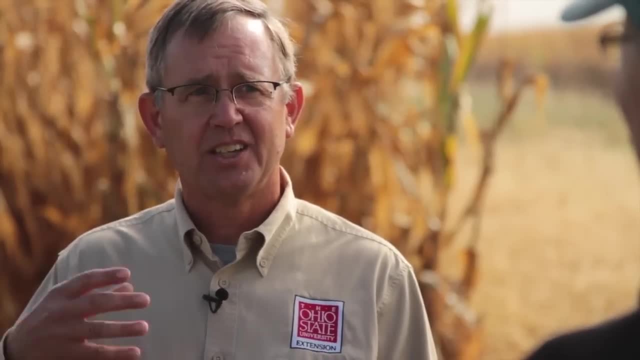 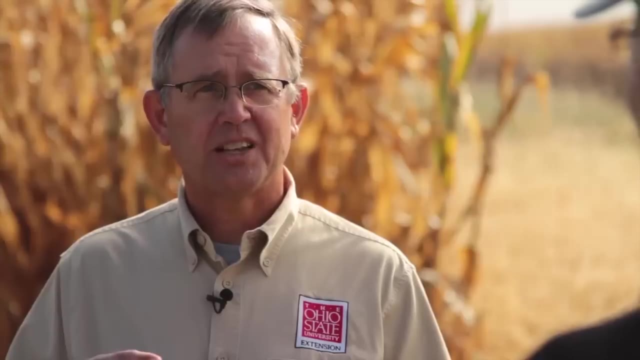 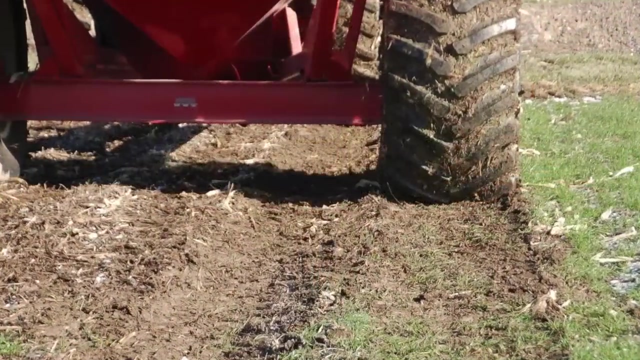 experiments here that are proving that. We have some compaction plots comparing subsoil steel versus living cover crops. We're purposely compacting these plots in the fall under moist soil conditions by using a grain cart and going back and forth over the plots and forcing that. 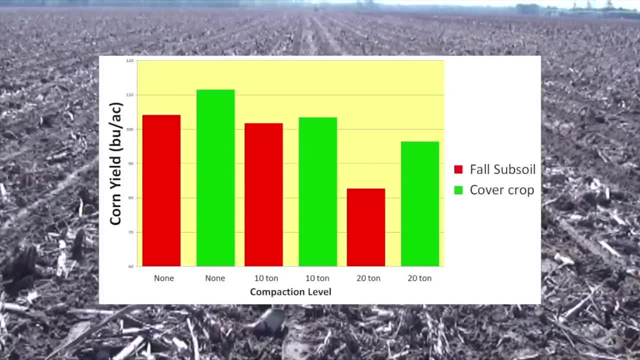 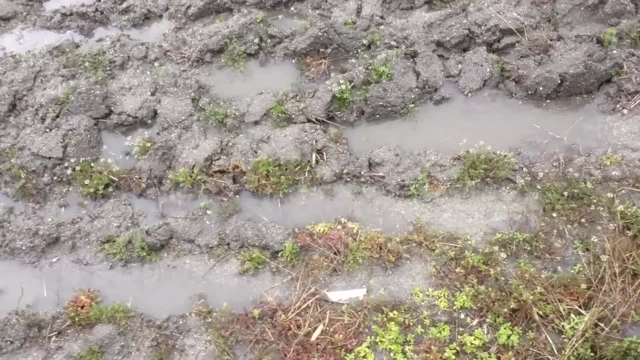 compaction And then the cover crops are planted and then we're comparing that to using a subsoiler and our yields are showing better results with the cover crops. And of course when you get some heavy range you can see staining water problems. you know that show up between the compaction levels of 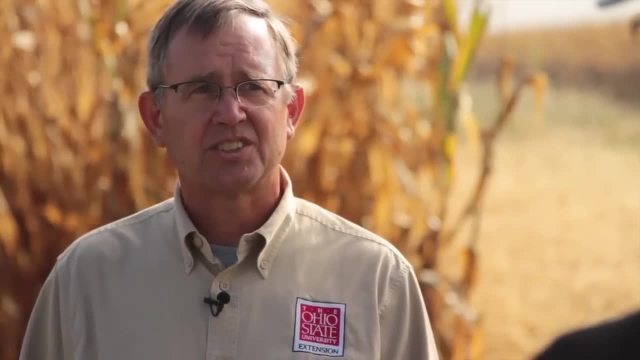 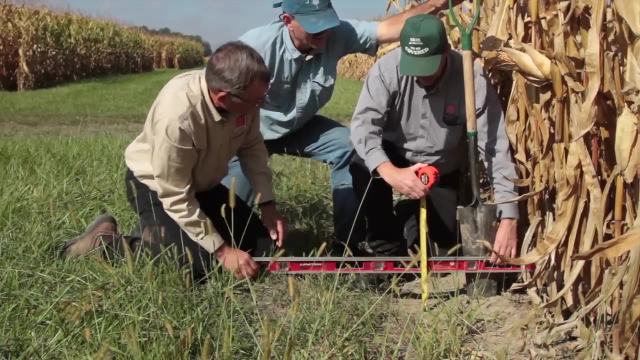 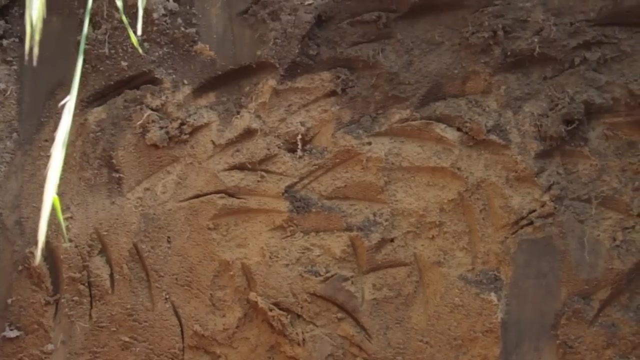 the plots also that way, And the cover crops are outdoing the steel. So what's the explanation for these rather surprising results? When you look at a soil, you have to look at the components, And the major component of most soil is sand, silt and clay. Now that makes up a 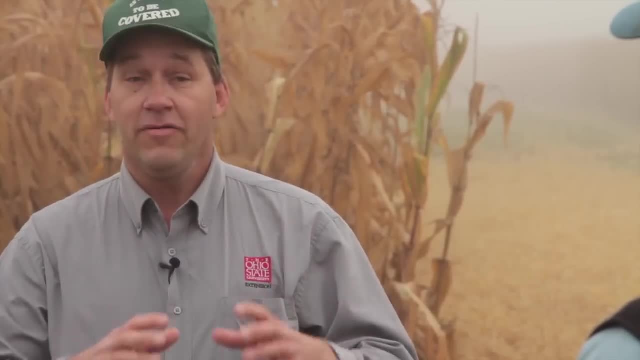 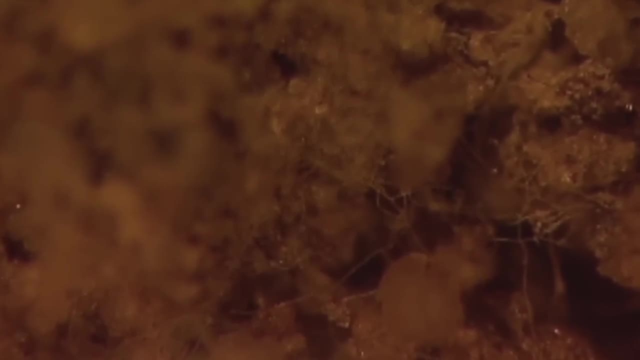 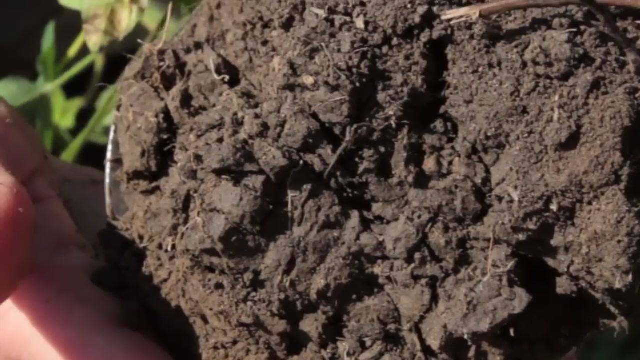 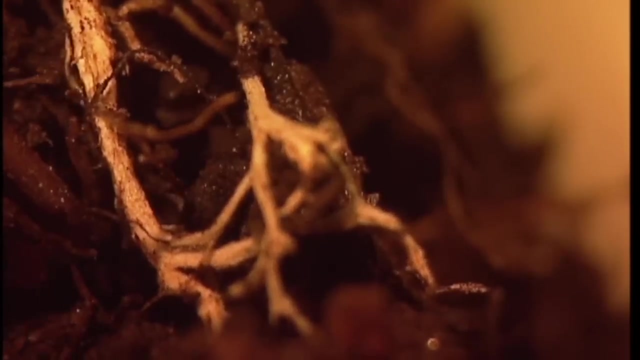 lot of the soil components. You know this is like regular soil. It's just going to get more and more, but it should be. you can't tell from the bottom of the soil. It should be organic. You know you have to. you know it's something you have to do to use the soil you have to use. the soil to get that organic matter out of the soil And you want to keep that organic matter and just use that organic matter for the soil. You want to use that organic matter and I've been going for some years now because I've only looked at soil and I'm like man, this is bad. It's just not working And I don't know how we'll do this. I don't know how much soil we need to be able to do. Yeah, I know, I know, 100 to 150 years through tillage. 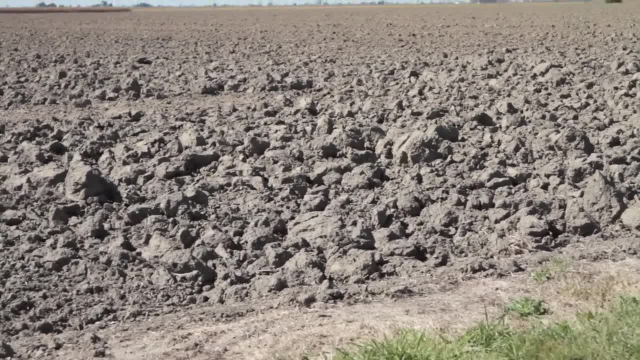 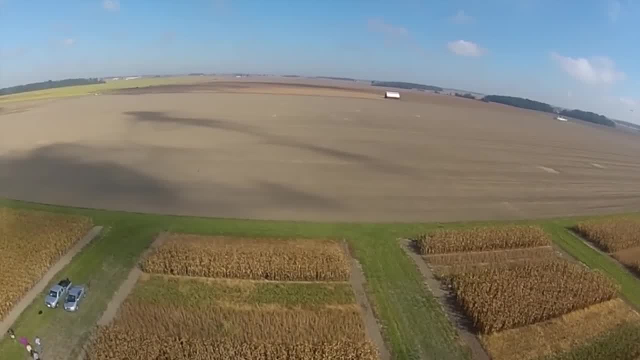 we've lost probably at least 60% of our organic matter. Some studies say as much as 80% of the organic matter is going right up into the atmosphere And this is a good area, because this was a black swamp in Northwest Ohio. 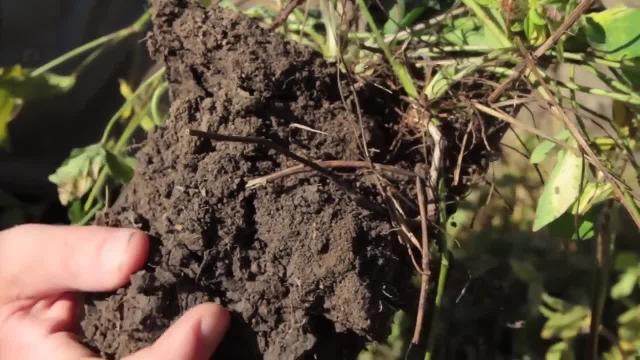 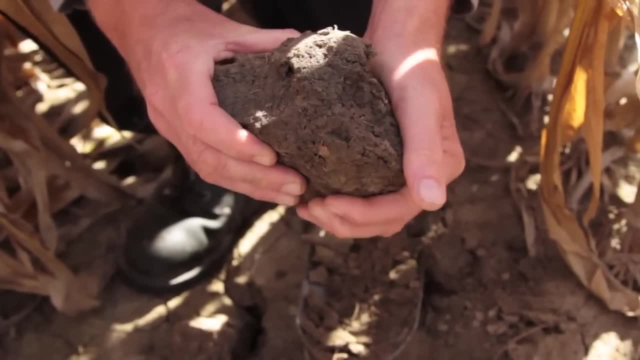 When the first settlers came here, they said our soil was as black as midnight. And when you look at the soil now, you'll see that it's not as black. it's actually kind of a brown. It's lost its color, so it's lost a lot of its organic matter. 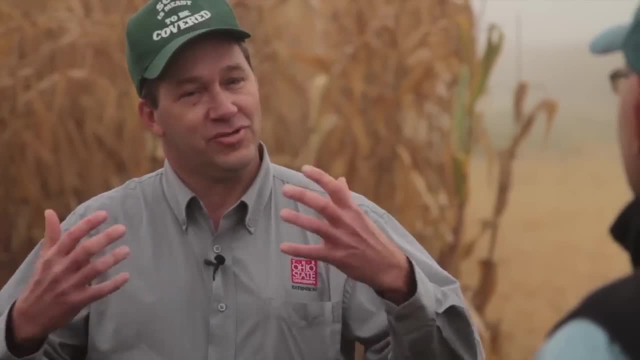 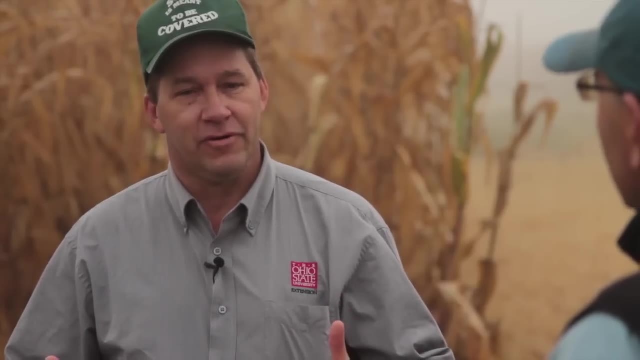 I like to tell farmers that a lot of times when you till the soil, you turn it into cement mix, And so the soil gets very hard and dense, And one of the things that we've learned is that if I was going to drill into cement, 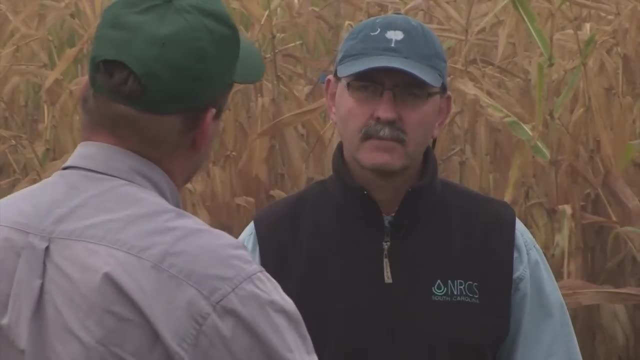 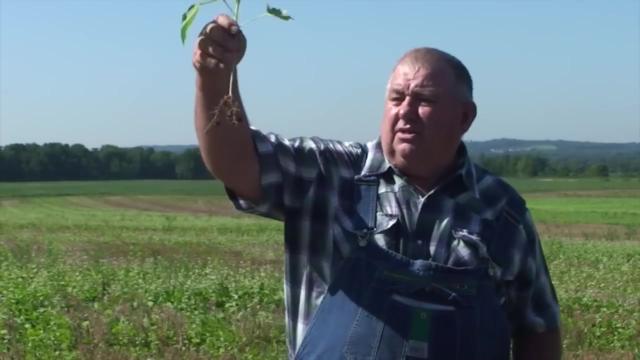 I would start with a small drill and then use a bigger drill to go through it, And so that's what we do with the cover crops. The cover crops actually have very fine roots and they form a small hole, And then we follow that with corn. 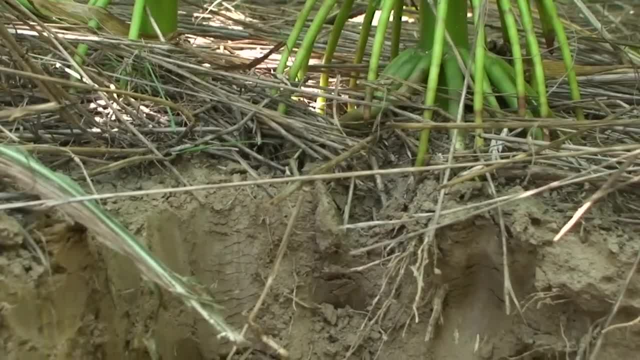 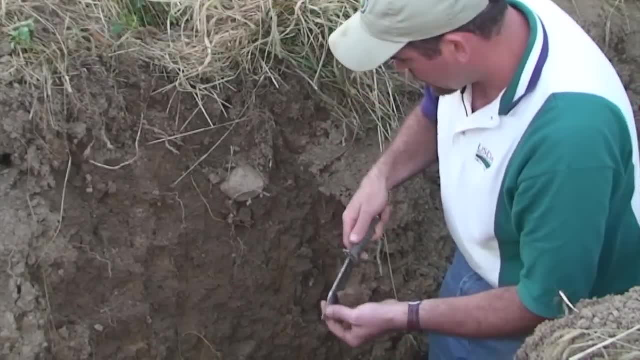 and hay, Corn and soybeans. and those corn and soybeans will follow those same channels down through the soil, And they also follow earthworm holes, because earthworms are fairly big and they're also enriched with nutrients And so those roots just really proliferate. 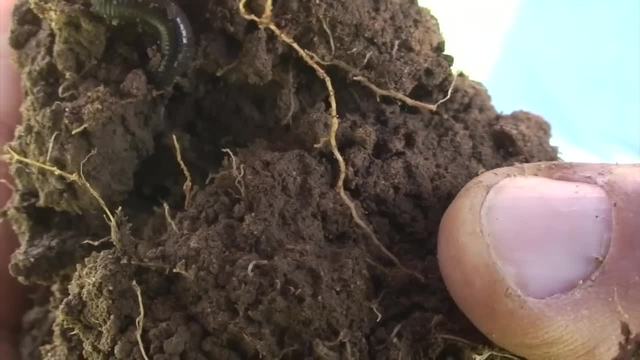 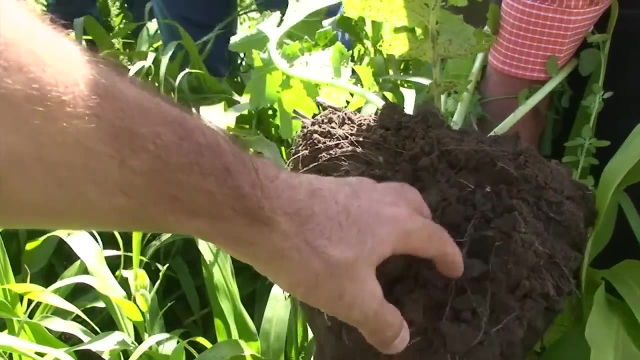 around those earthworm holes And that's how we then can actually loosen the soil up, is it's the roots that loosen the soil up and give that carbon to the soil, and also is a storehouse for all the nutrients in the water. 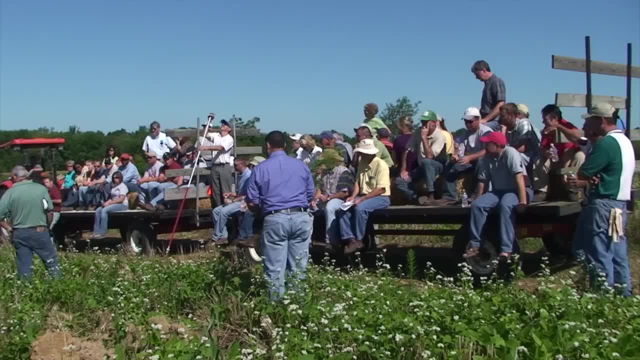 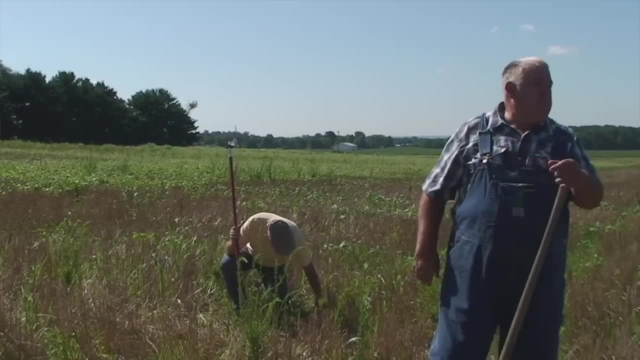 So a lot of innovation is happening. It's really an exciting time because farmers are seeing that hey, there's different ways we can improve our soils: by adding cover crops, by not going to steel, by reducing our tillage. A lot of good innovative thinking, I think, is happening. 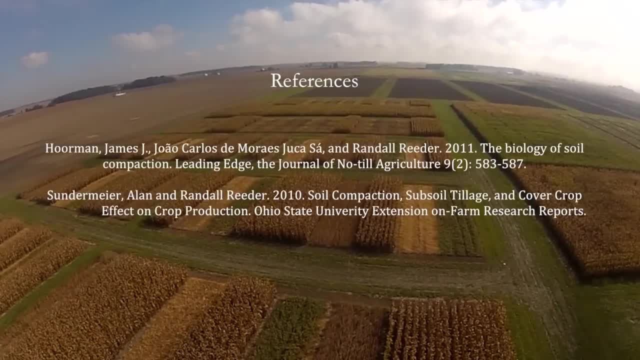 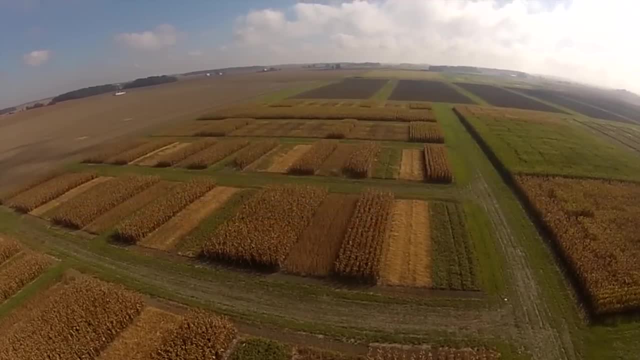 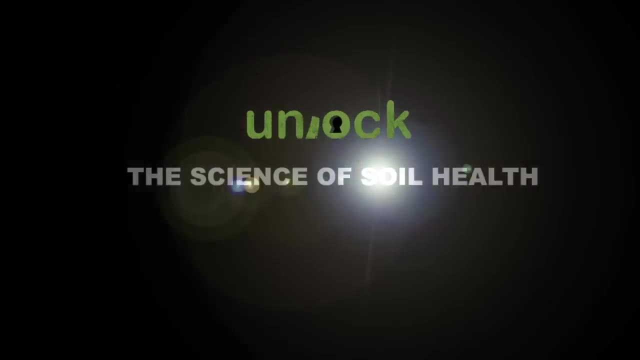